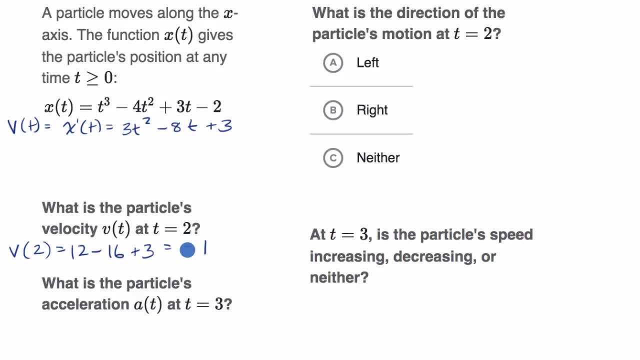 You might also be saying: well, what does the negative mean? Well, that means that we are moving to the left. Remember, we're moving along the x-axis, So if our velocity is negative, that means that x is decreasing or we are moving to the left. 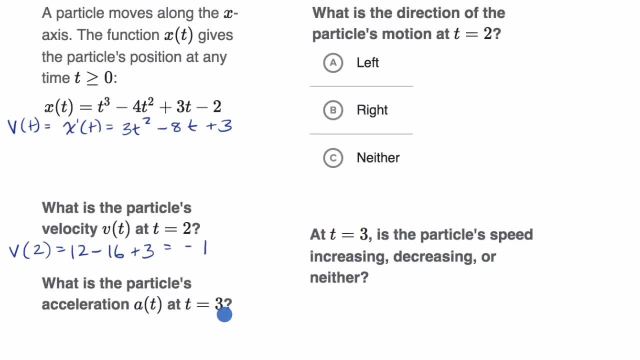 What is the particle's acceleration? a of t at t equals three. So pause this video again and see if you can do that Well here. the realization is that acceleration is a function of time. It's just the derivative of velocity, which is the second derivative of our position. 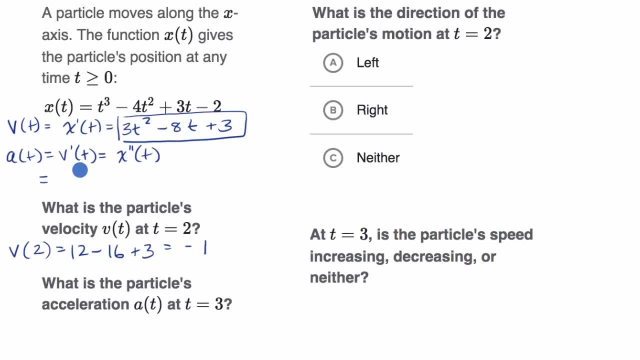 which is just going to be equal to the derivative of this right over here. And so I'm just going to get: derivative of three t squared with respect to t is six t, derivative of negative eight t with respect to t is minus eight, and derivative of constant is zero. 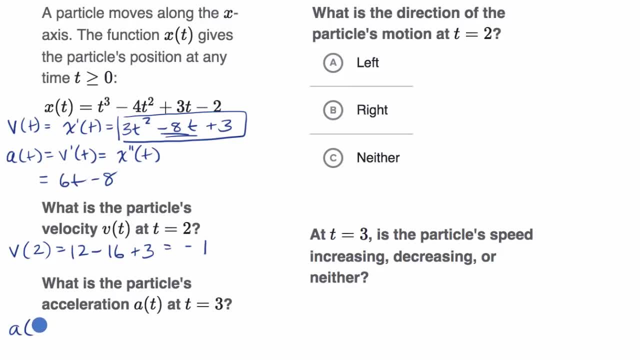 So it's just going to be six t minus eight. So our acceleration at time t equals three is going to be six times three, which is 18 minus eight. So minus eight, which is going to be equal to positive 10.. All right? now they ask us: 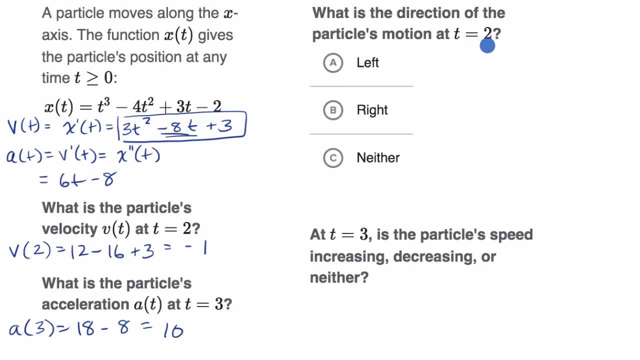 what is the direction of the particle's motion at t equals two? Well, I already talked about this, but pause this video and see if you can answer that yourself. Well, we've already looked at the sign right over here, The fact that we have a negative sign on our velocity. 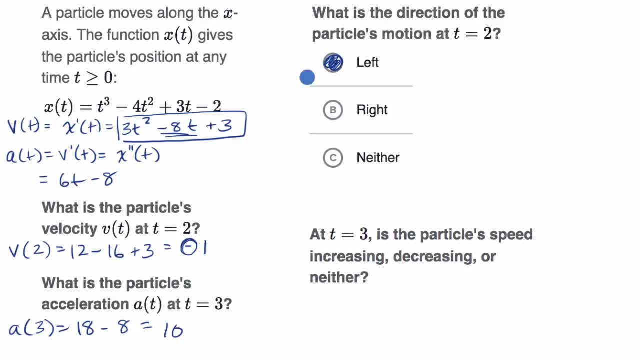 means we are moving towards the left, So I'll fill that in right over there At. t equals three. is the particle's speed increasing, decreasing or decreasing, Increasing or neither? So pause this video and try to answer that. All right, now we have to be very careful here. 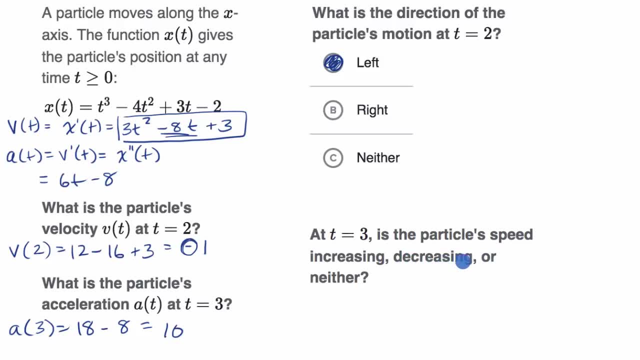 If it says: is the particle's velocity increasing, decreasing or neither, then we would just have to look at the acceleration. We see that the acceleration is positive, and so we know that the velocity is increasing. But here they're not saying velocity, they're saying speed. 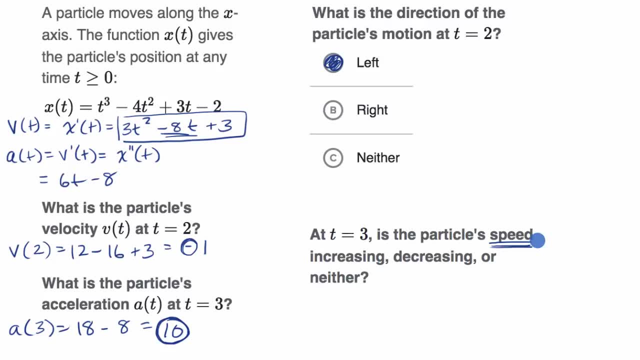 And just as a reminder, speed is the magnitude of velocity. So, for example, at time t equals two, our velocity is negative one. if the units were meters in second, it would be negative one meters per second, But our speed would just be one meter per second.